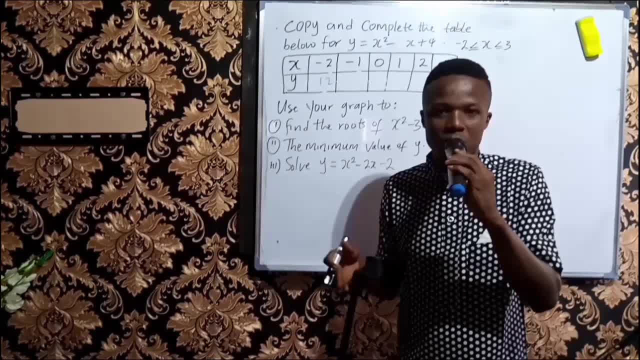 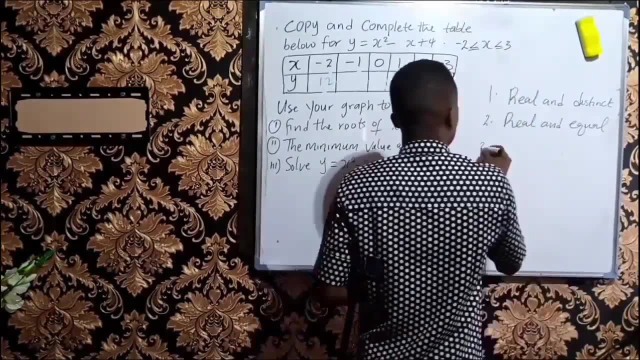 of nature. The nature of roots of quadratic equation can be in three categories, which I will write on the board now. So you can now see that the roots of a quadratic equation can be written in three categories. The roots of a quadratic equation can be written in: 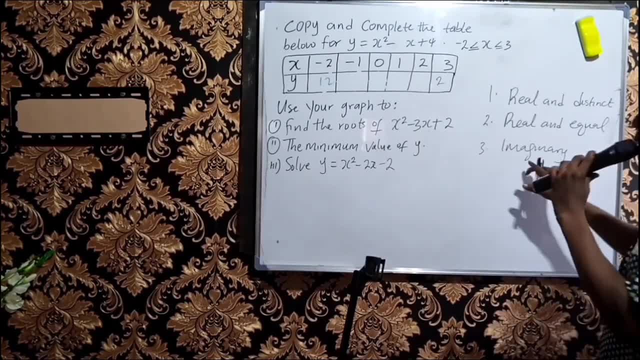 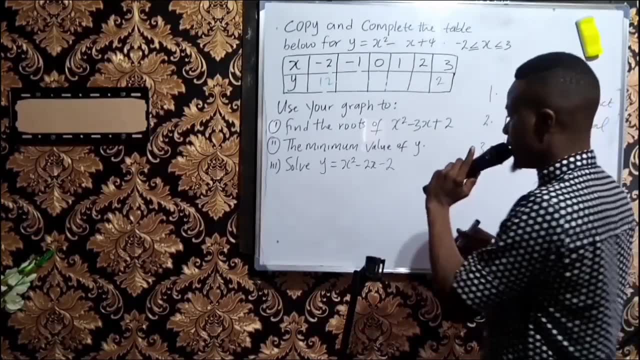 three categories. The roots of a quadratic equation can be written in three categories. It can be real and distinct. It can be real and equal, or imaginary, as the case may be. So let me exemplify this for you on the board. Okay, for it to be real and imaginary, let's. 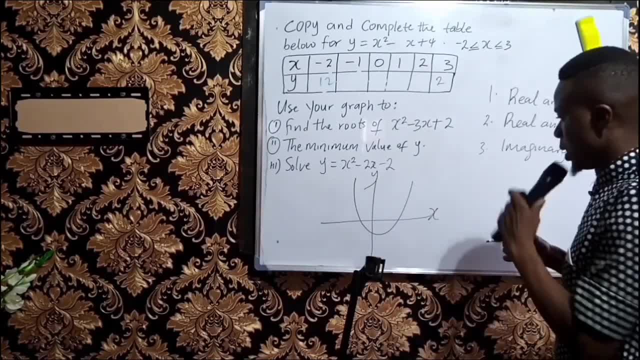 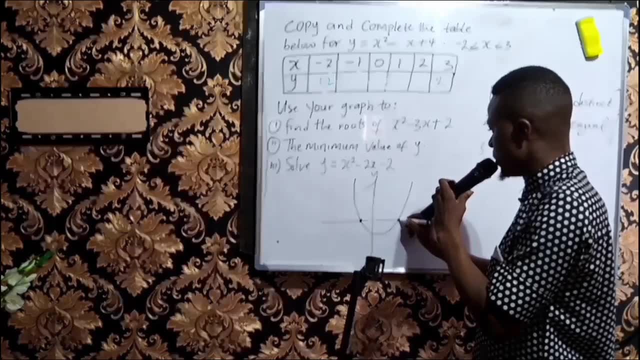 say, you have something like this. A clear look at this curve or graph will tell you that the curve is touching the x, as it is at two different points and these are real values of x that will satisfy this quadratic equation and they are at two different. 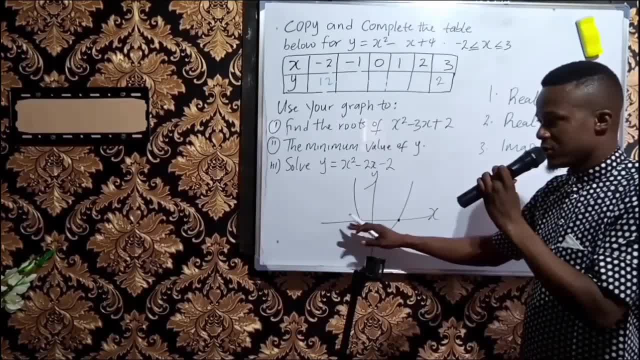 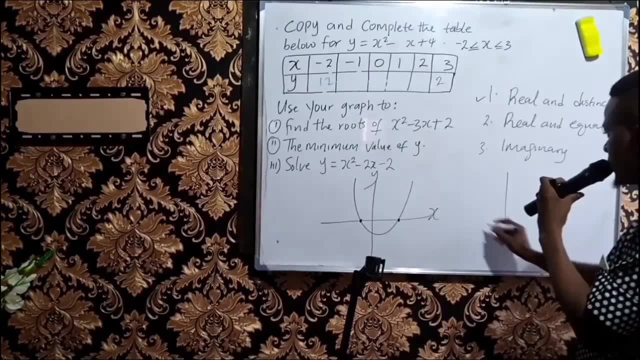 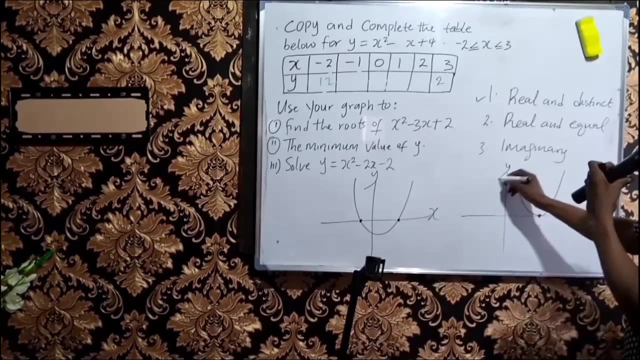 points, which means the values of x. here are two different values. So we say the roots here are real but distinct. Sometimes you can have a curve that looks like this. You will see that the curve is just touching the x-axis at only one point, unlike this one. 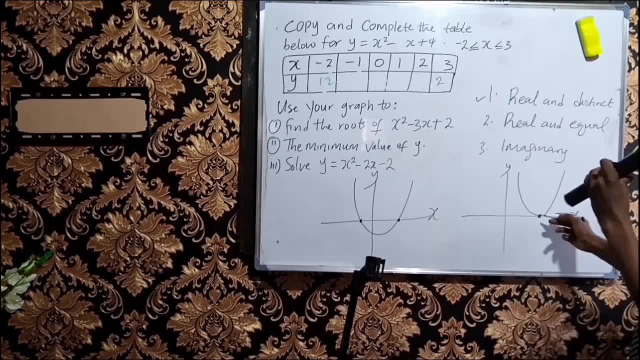 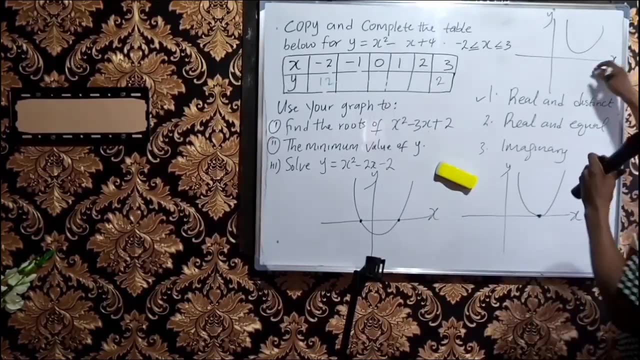 where it touches it at two different points. So if this happens, we say that the roots of this quadratic equation are real, but equal because they lie at the same point. Okay, what if you have some curve that looks like this: Yeah, you have your x and y-axis At. 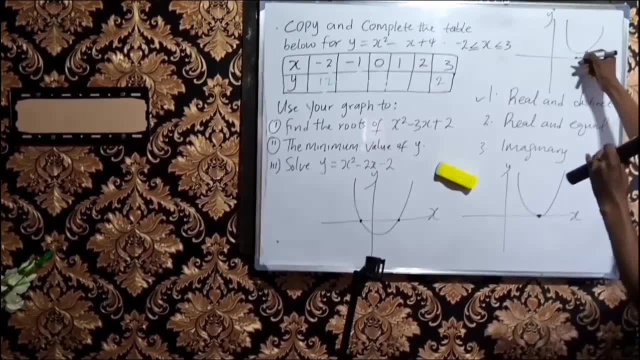 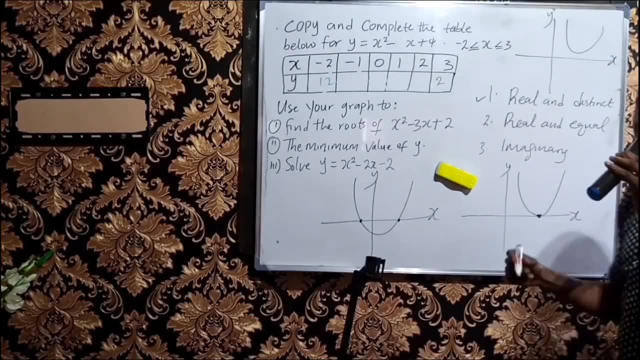 this case, there is no point at all where this curve is touching the x-axis. Because of that, we say that the roots are imaginary, because no real value of s can satisfy that particular quadratic equation. Okay, now let's go to the main business. 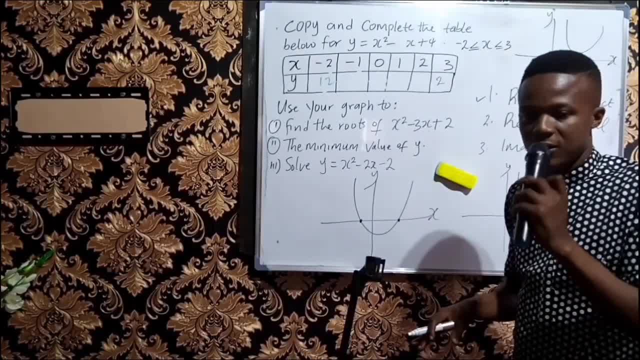 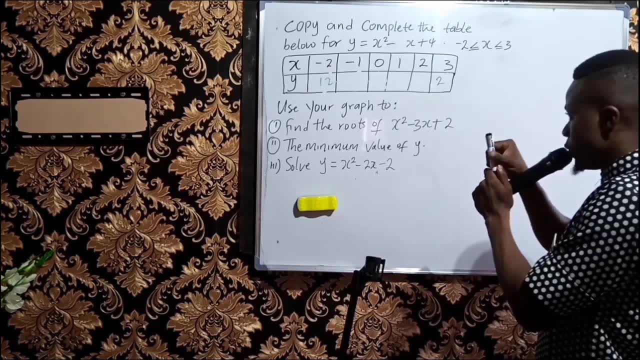 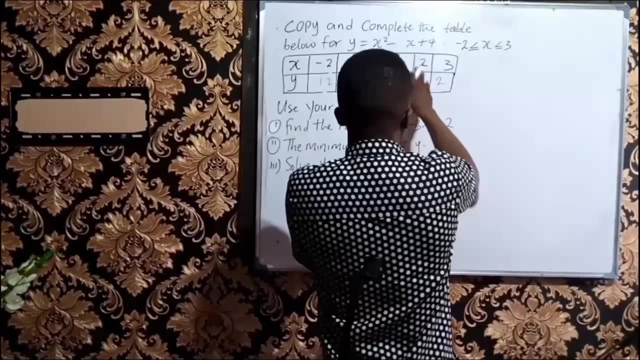 The equation was x here, So let us tackle it together. To continue to solve this using graph to solve quadratic equation implies that you have to first of all make out a table of values. That is why we have to copy and copy, So you have to make a table of values. 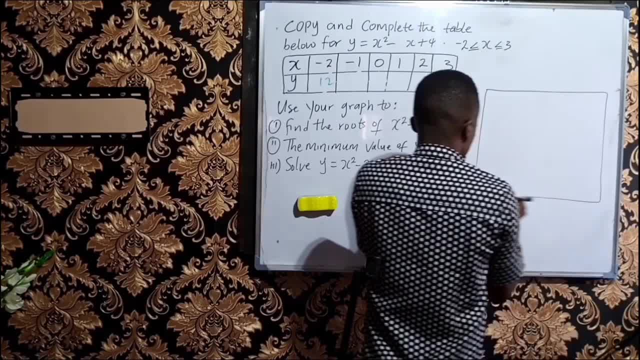 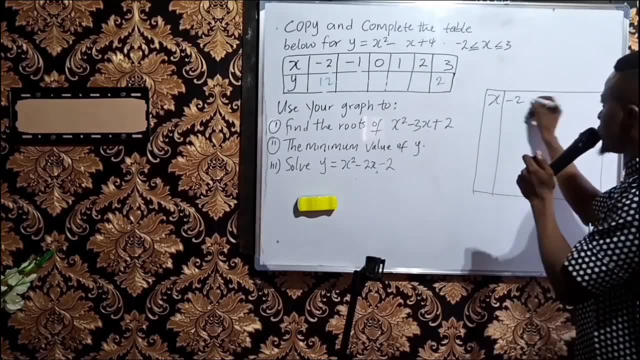 like this, And that is exactly what I'm doing now. You have the values of x and the values of y, So you have to make a table of values like this, And that is exactly what I'm doing now. So the values of our x range from: uh, we have minus 2.. We can still have. 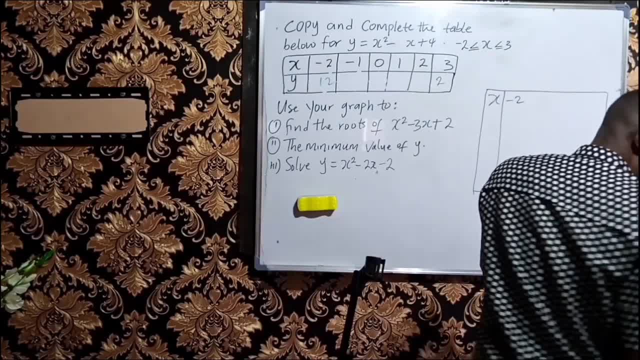 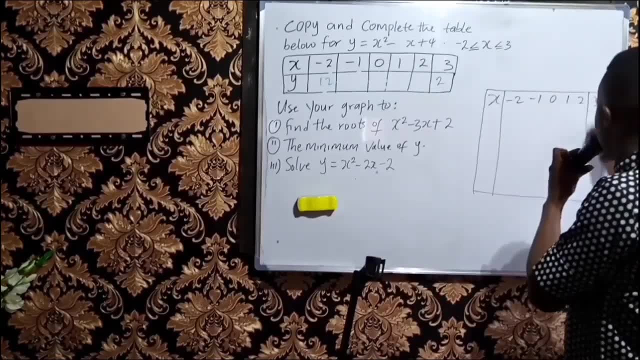 uh, not just minus 2. there are so many values of x We have minus 2, have, uh, minus 1.. We have 0.. We have 1.. We have 2 and 3.. So these are the values of x that are given to us. 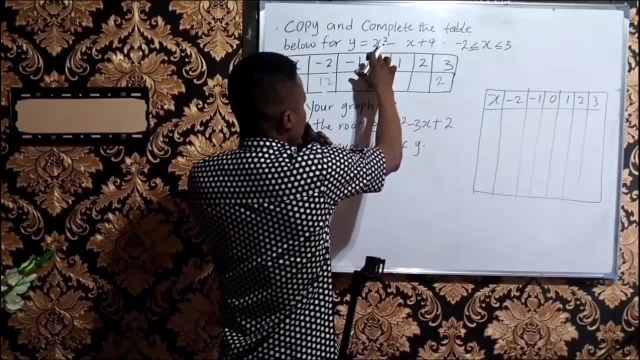 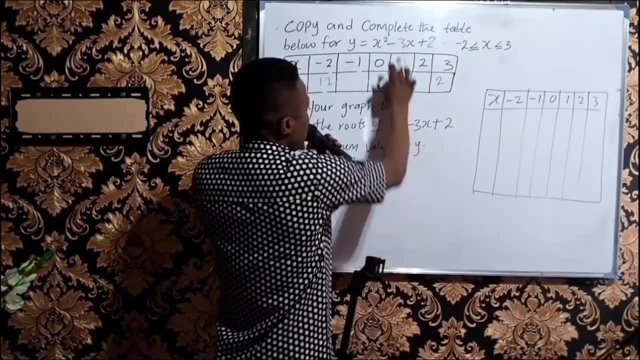 So, after writing out these values of x, the next thing you write is the first element of the quadratic equation. The quadratic equation is 3x plus 2, okay, so x squared minus 3x plus 2. so the first element here is x squared. you plug in x. 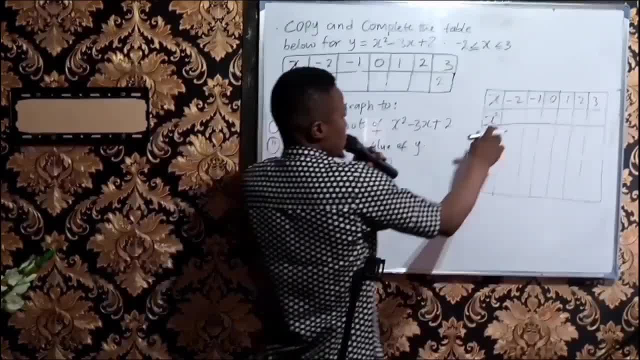 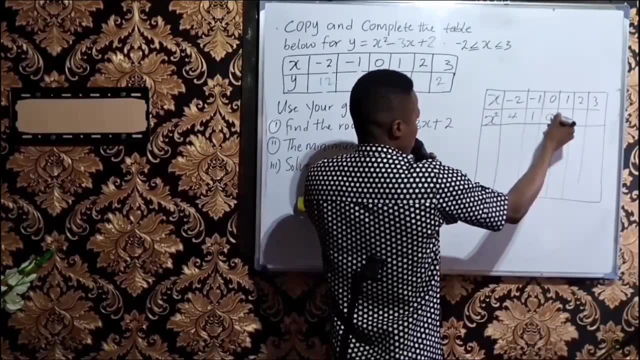 squared um x. squared means you are squared in the values of x. so you say: minus 2 squared is 4. minus 1 squared is 1: 0 squared is 0, 1 squared is 1, 2 is 4 and 3 is 9. the next thing there is: 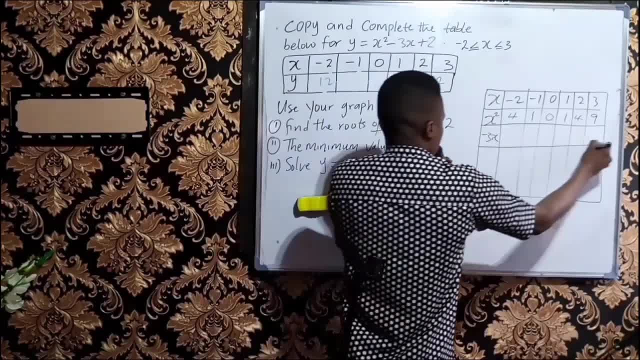 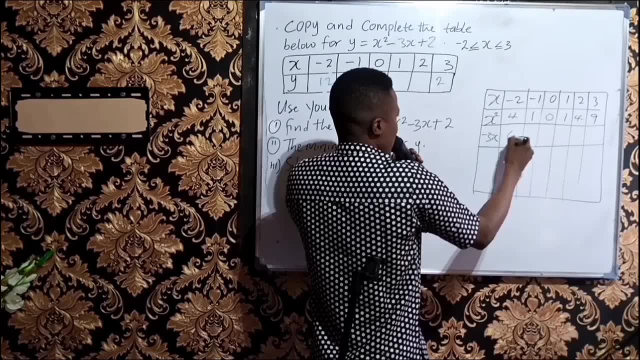 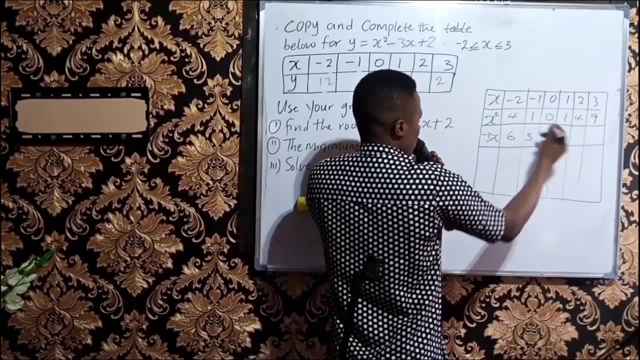 minus 3x. minus 3x implies you are multiplying the values of x by minus 3. so minus 3 times minus 2 is 6. minus 3 times minus 1 is 3. minus 3 times 0 is 0. we have minus 3 minus 6 and minus 9. 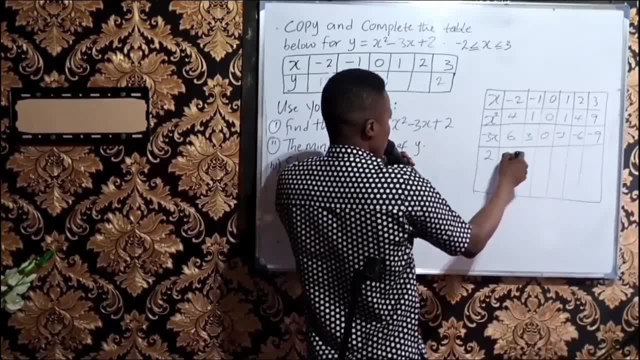 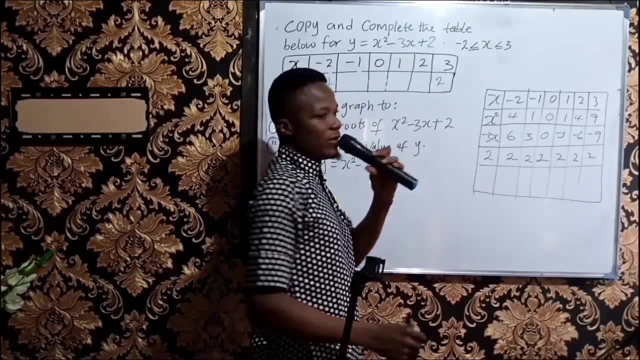 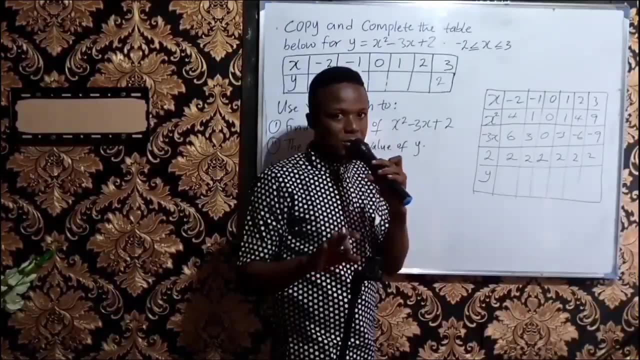 then, finally, we have a constant. 2 plus 2 means that you repeat 2, because a constant remains the same. it doesn't change. having written the constant, you've got to write the values of y. so you can see the procedures i'm following to be able to fill in this table of values now, as you want to. 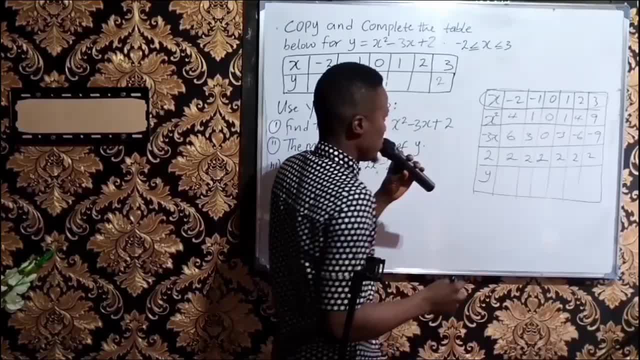 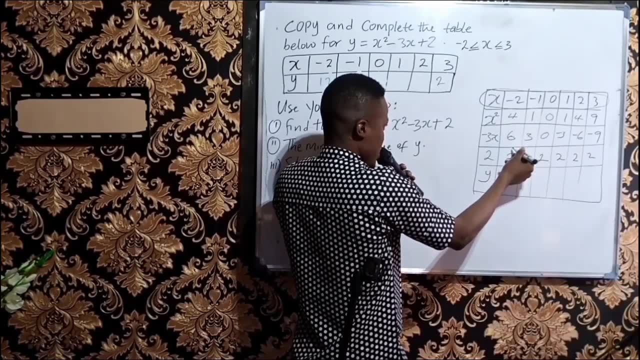 add up. don't include this, because this is not part of the quadratic equation. the quadratic equation began from x squared, so you start from x squared, which is 4 plus 6 is 10, 10 plus 2 is 12. that is why we're having 12 here. they did that one for us. 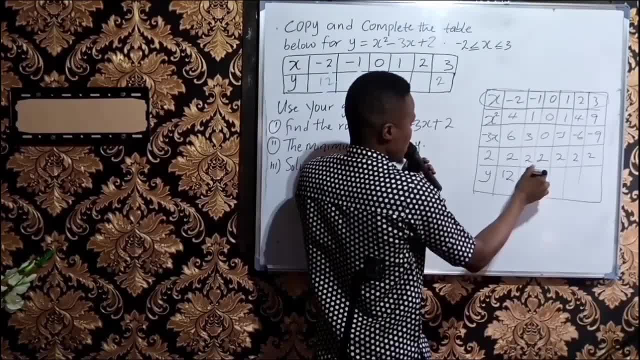 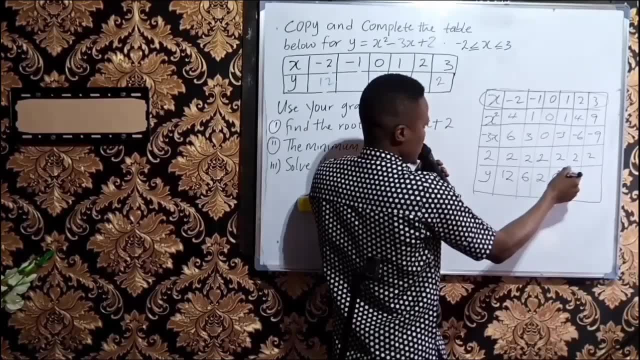 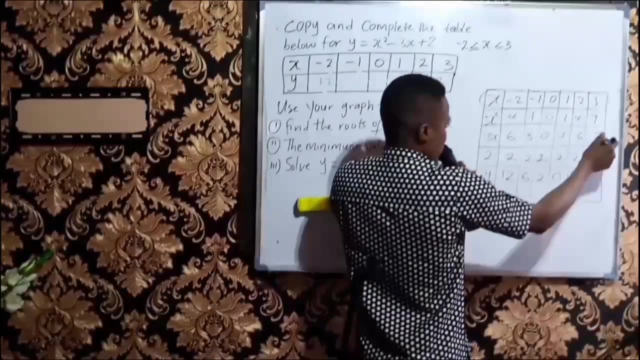 1 plus 3 is 4, 4 plus 2 is 6, 0 plus 0 plus 2 is 2.. 1 minus 3 is minus 2, minus 2 plus 2 is 0,. 4 minus 6 is minus 2 minus 2 plus 2 is 0, and 9 minus 9: 0, 0 plus 2 is 2.. 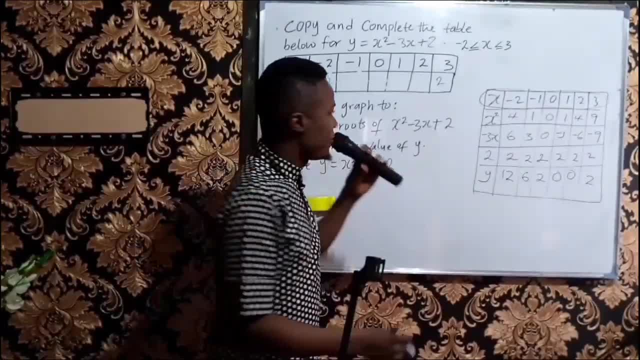 so we have carefully made out values for y, easy way, easy pattern. then you now fix it in here to complete the table. here is 6, here is 2, 0, 0, 0, 0.. Now just want to point each of those values equal 0, 0 and 0.. for each other to complete, as you might have, which is x, x plus x, you, with respect to, and find each of these models with these values. 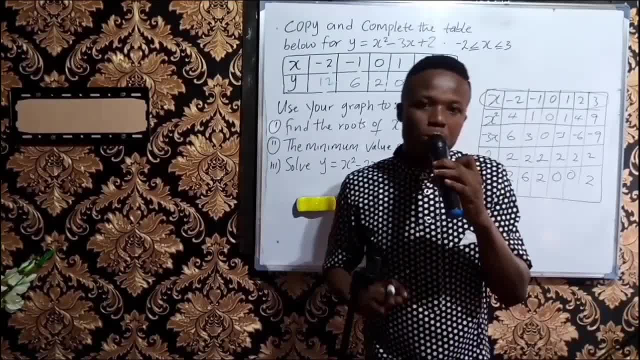 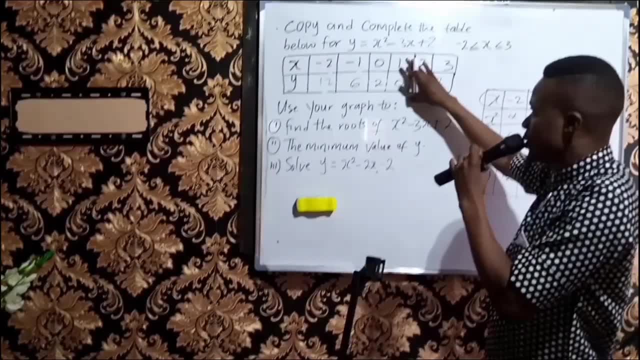 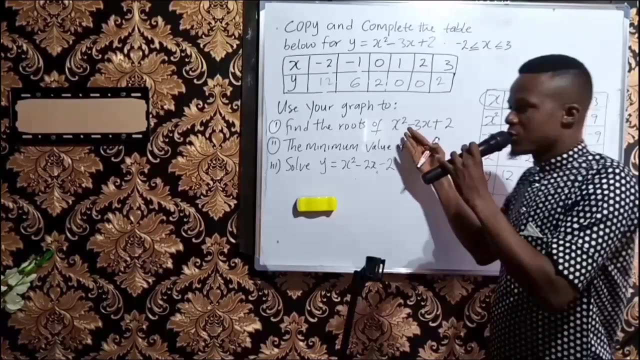 and 2 is already here. this is how to copy and complete a table. once you've copied and completed a table, the next task that follows is to use this table of values you've completed to draw the graph, and from the graph we'll be able to find the roots of this quadratic equation. the roots of the quadratic. 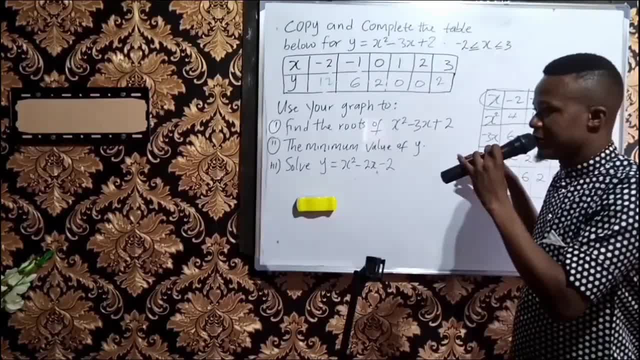 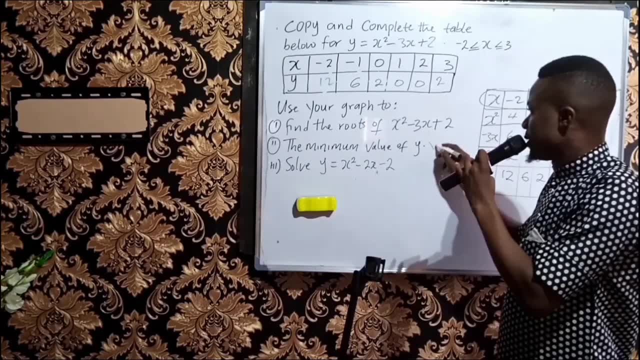 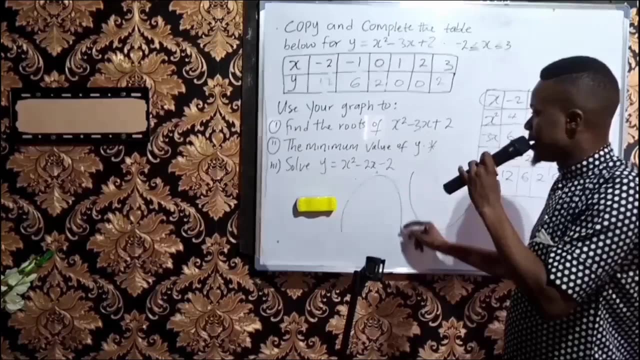 equation are just the points where the curve you must have drawn. we touch the X as X the minimum value of Y. okay, this is not part of the equation, but minimum value is obtained when the curve slopes downwards like this. if slopes like this, it is going to have a maximum value, because here is maximum, while here is a. 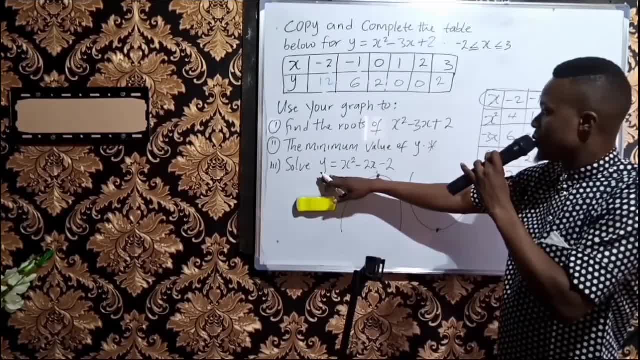 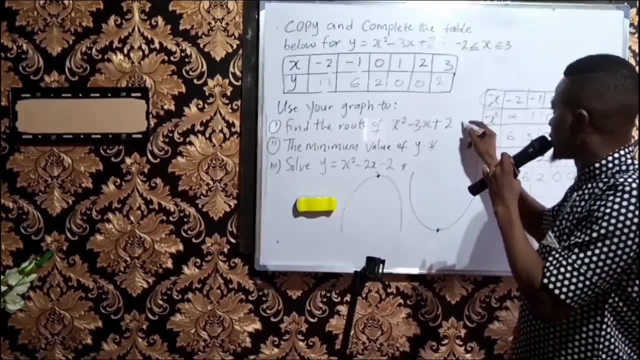 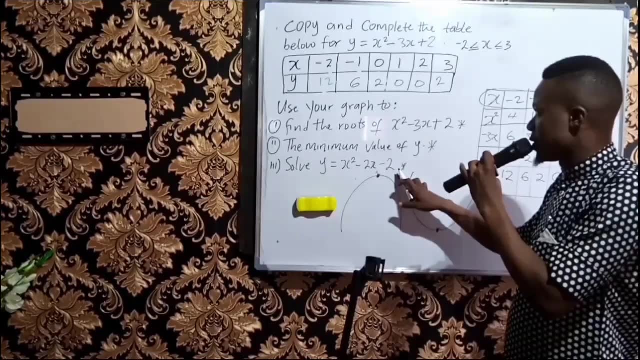 minimum. then we are also asked to solve the equation where you have Y, is X squared minus 2, X minus 2. remember: this equation and this equation are entirely two different equations. but with the aid of quadratic equation graph, we can solve a different equation from the graph we've made. so let us see how it goes. okay, at this point we have 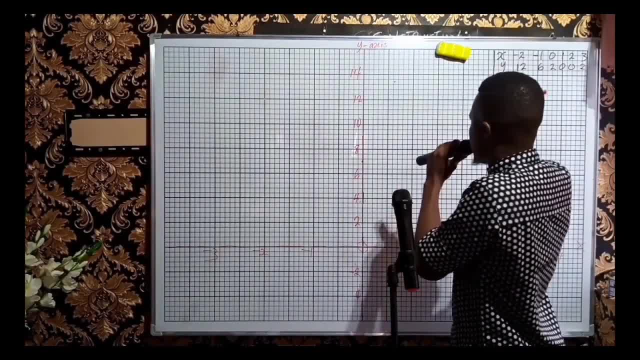 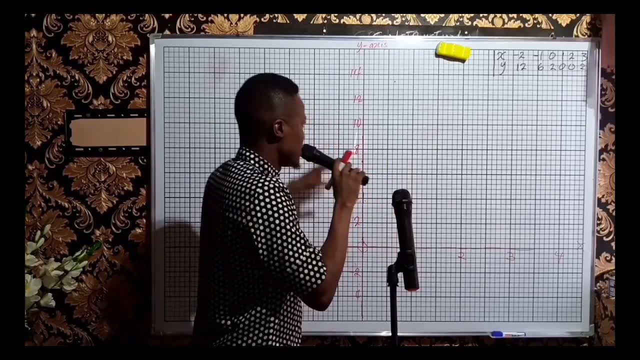 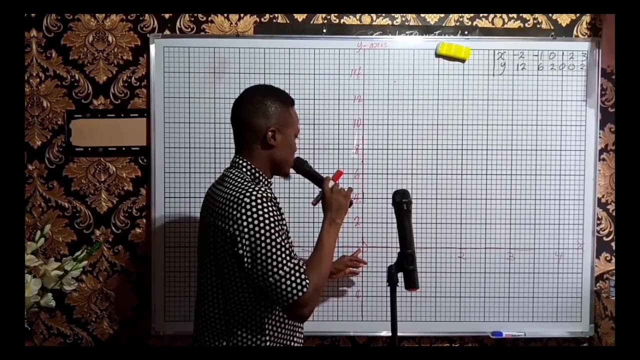 successfully made the table of values, so we are not going to use this table of values to plot the graph. to plot this graph, we have carefully written out the axis of Y and the axis of X, and in the axis of X I made it in such a way that: 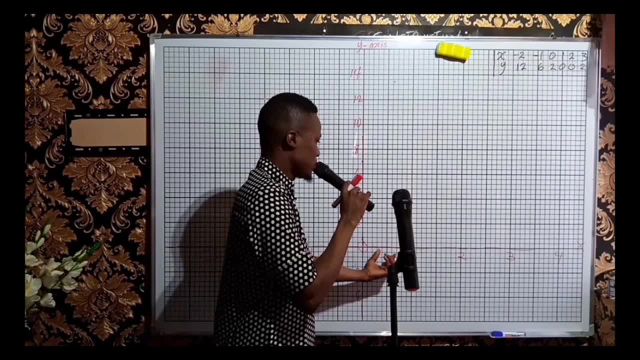 I'm using I'm jumping to the X axis of Y and the X axis of Y and the X axis of X, and in the axis of X I made it in such a way that I'm using I'm jumping to two boxes to get one unit: 2, 3, 4, etc. but in the values of X I'm just jumping one. 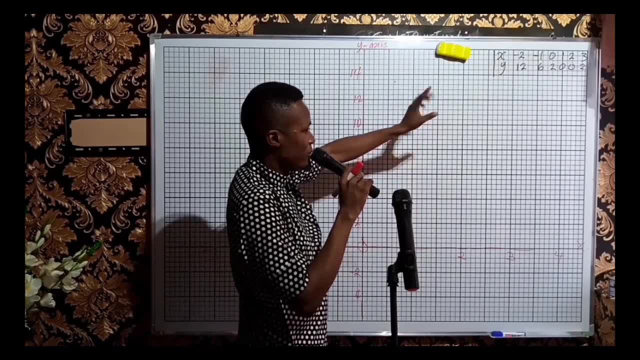 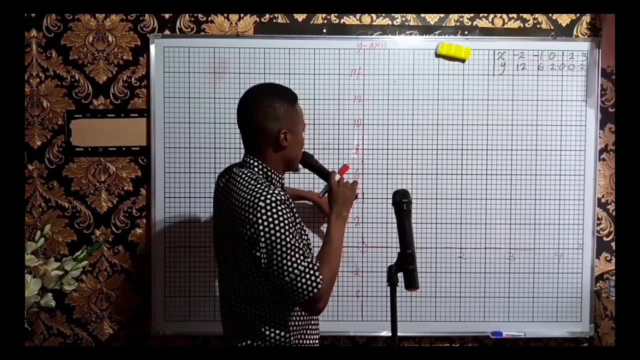 box to have two units. this is dependent on the kind of values I have for X and Y, for example, the values of Y are too big, up to 12, and if I write 1, 2, 3, the graph may not contain it. but the values of X are too small. and here, because I'm 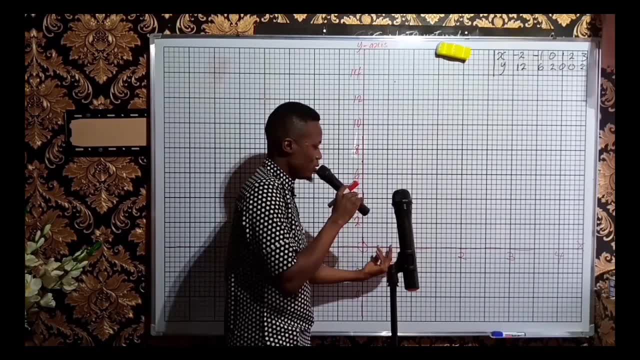 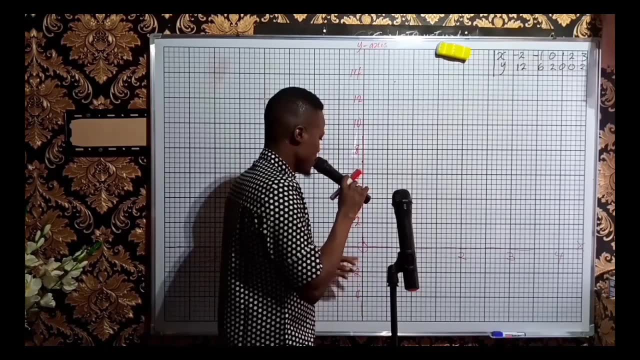 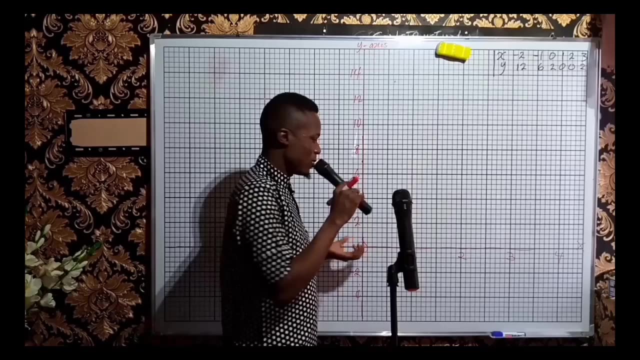 jumping two boxes to have one unit. I'll call it 2 cm to 1 unit. as we now write in 5, 10, 15, it will be 2 cm to 5 units. here I'm jumping one box to write 2, it will be 1 cm to 2 units, because one box is just 1 cm. okay, now, at this point, let 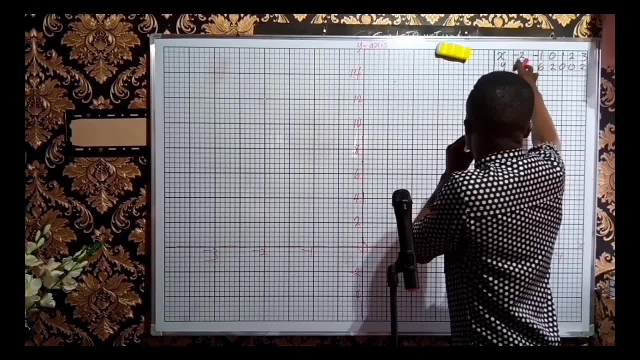 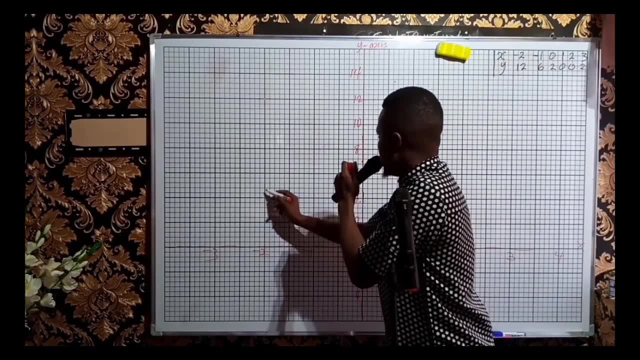 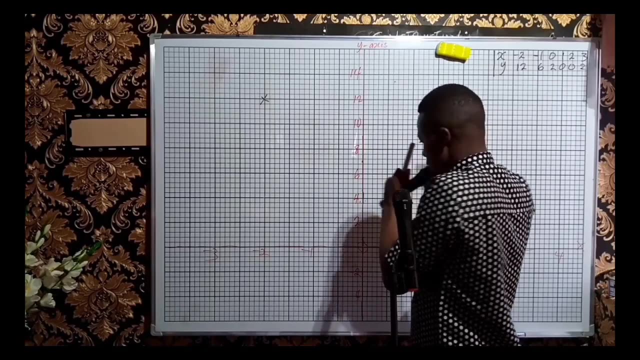 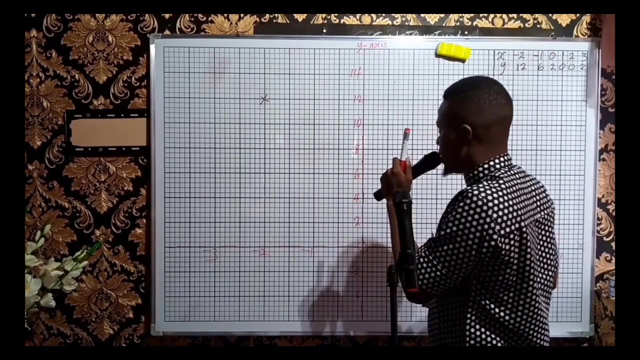 us proceed to plot the graph. when X is minus 2, the value of Y is 12. so here you look at the line of 12, you trace it. so you are plotting somewhere here. okay, so you have minus 2 for X and 12 for Y. then the last thing you do again is you have: 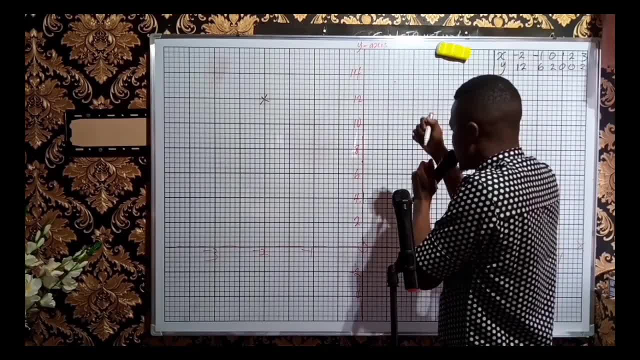 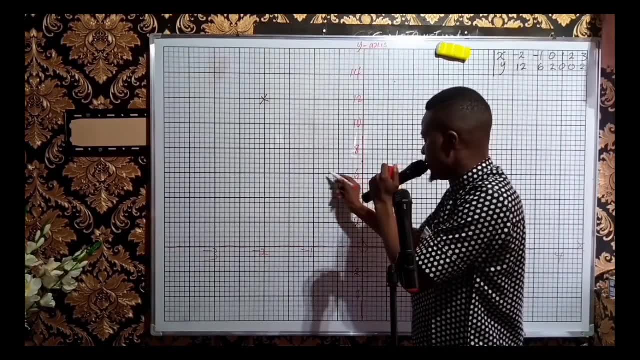 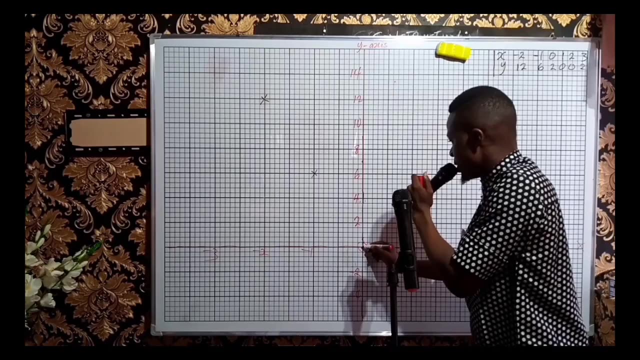 X as minus 2 and Y is 6. so X as minus 1 and Y is 6. look at X minus 1. here was this: look at where you're having 6. you look at where you're having 6. you look at where you're having 6. you mark another act. you have X: 0 and Y is 2. X is: mark another act. you have X: 0 and Y is 2. X is mark another act. you have X: 0 and Y is 2. X is 0 and Y is 2. you mark another one. 0 and Y is 2: you mark another one. 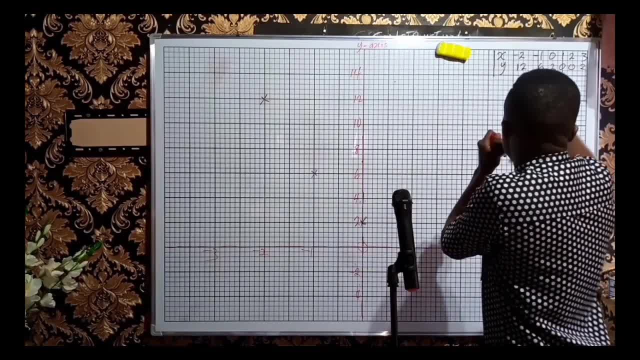 0 and Y is 2, you mark another one here at this point. when X is 1, Y is 0. when X- here at this point- when X is 1- Y is 0. when X- here at this point- when X is 1, Y is 0. when X is 1, Y is 0. so it's at this point. 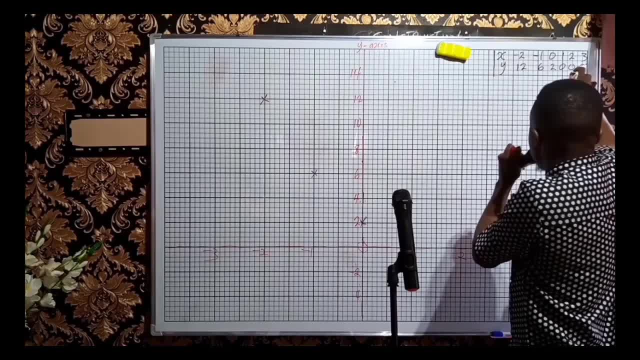 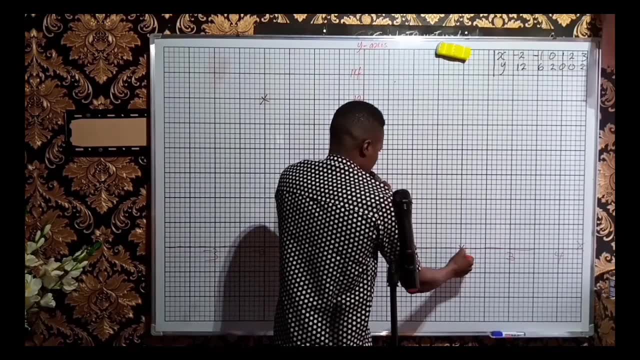 is 1, Y is 0, so it's at this point is 1, Y is 0, so it's at this point. you mark: when X is 2, Y is 0, also X is 2. you mark: when X is 2, Y is 0, also X is 2 here. look at X at this point. 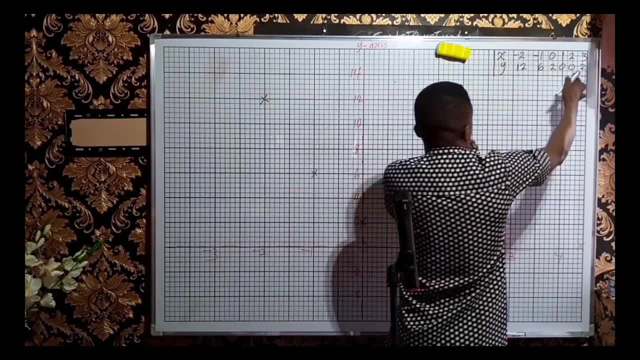 you mark: when X is 2, Y is 0. also, X is 2 here. look at X at this point, then after that you have that when x is 3, y is 2. when the value of x is 3, you have your y as 2. 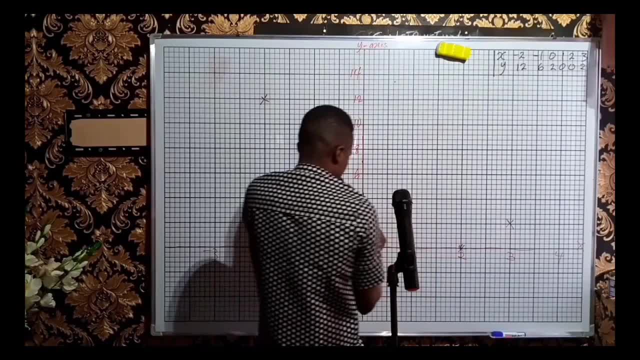 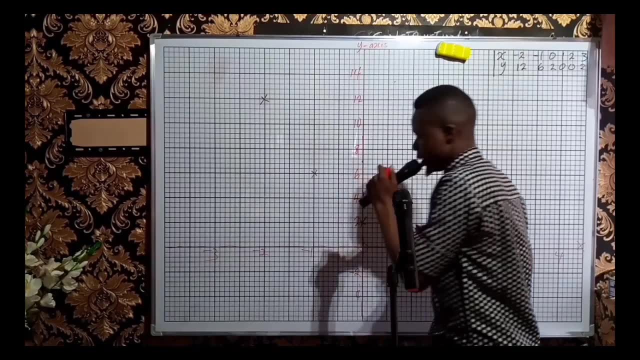 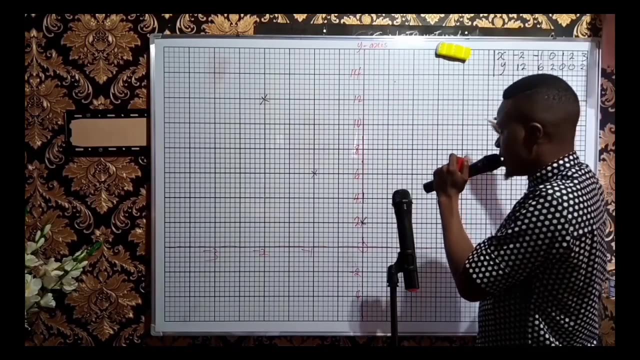 so that is it here. at this point, you might, because this is y here at 2 and the value of x is 3. okay, having done that, the next thing you do is to successfully join the points you've plotted together. okay, carefully, but you have to use a french curve. 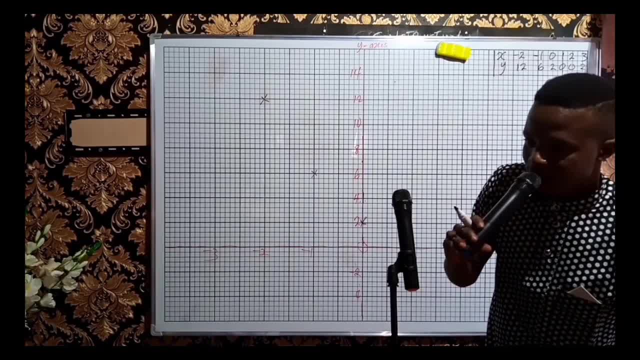 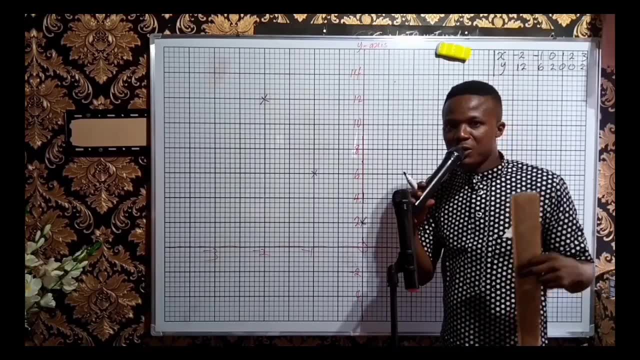 to do that. but since you're not having a french curve, i don't have it here, so i have to use my lula to do that. but you don't use lula to do that, you have to make use of a french curve, okay, or you? 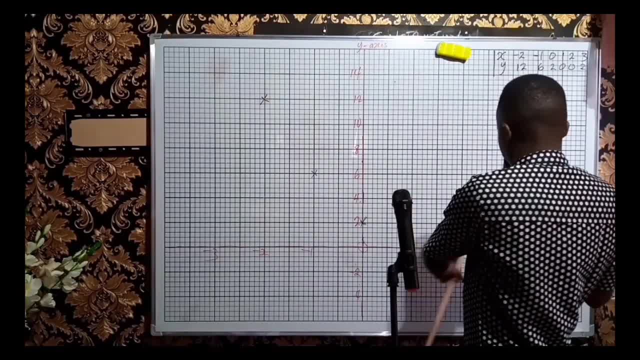 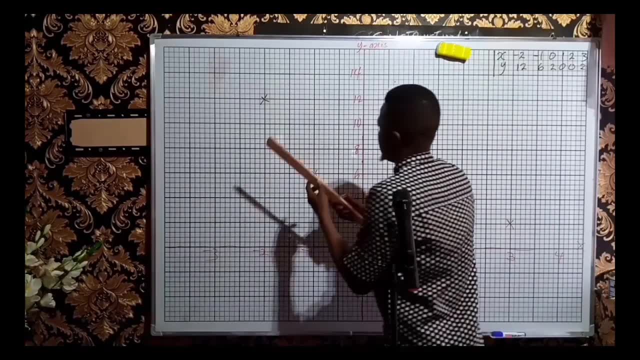 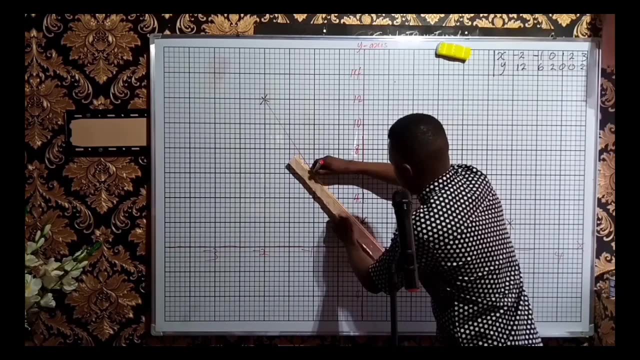 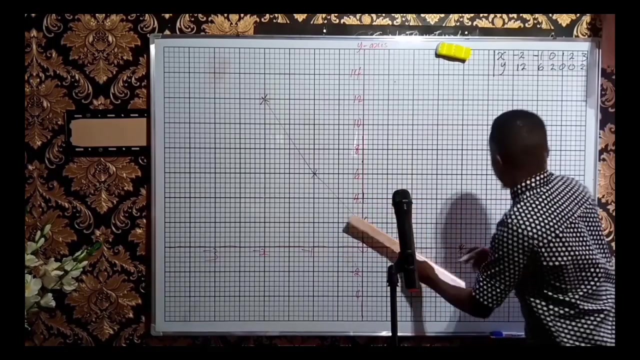 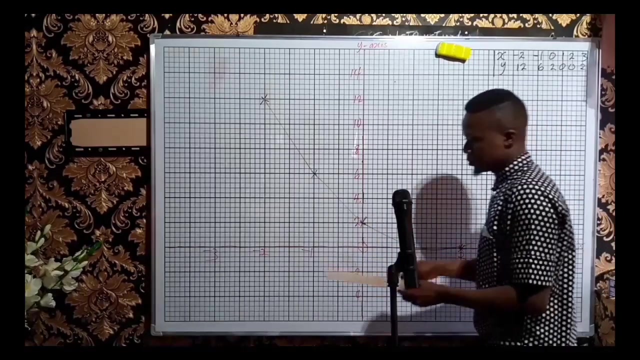 can get a broom, a soft broom, and bend it to the shape of this curve you've made and join it together. so let's see so, but this thing i'm doing you don't do that, but i don't have the option now. okay, normally you don't use lula to do this, but because i don't have the lula, 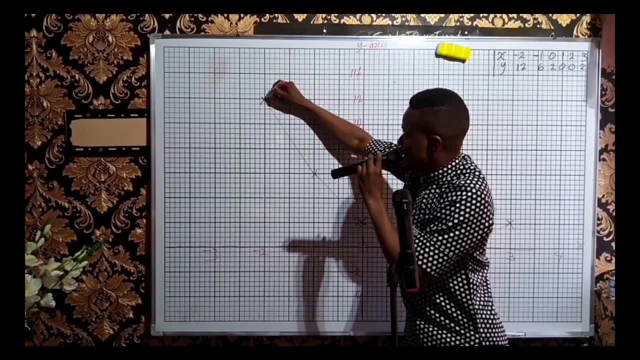 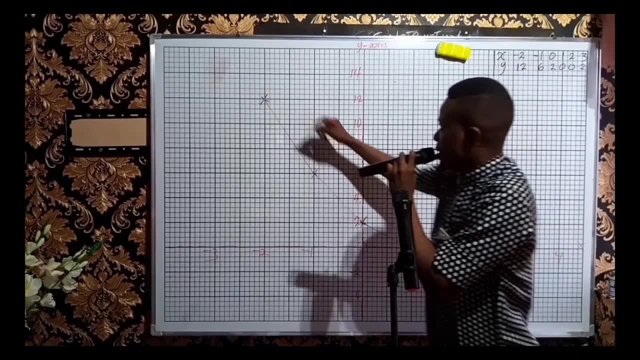 that is why- okay, normally you don't use lula to do this, but because i don't have the lula, i have used. i don't have the french curve here. that's why i used the ruler to join the lines and, as you can see, it is so straight, so i've joined the curve together and form something. 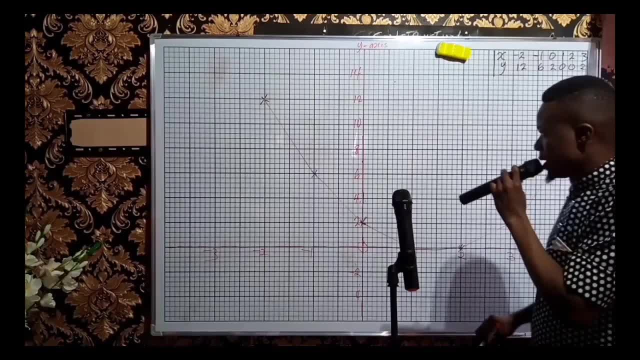 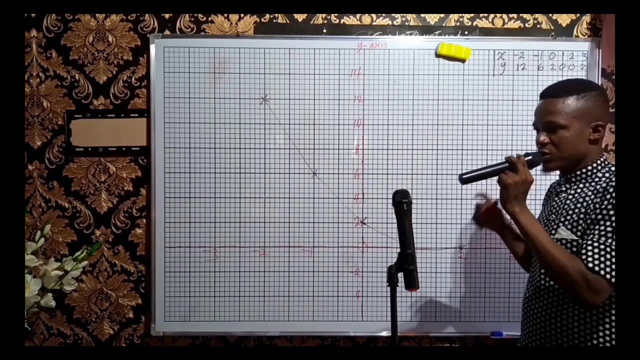 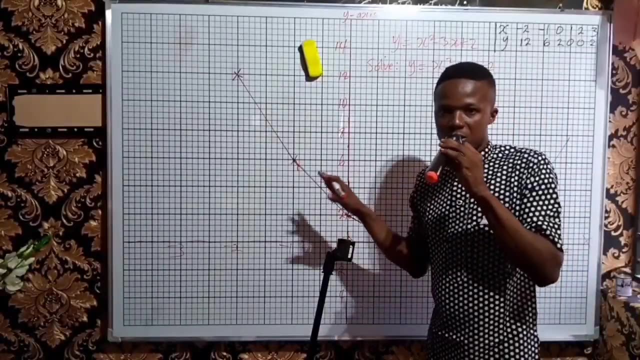 that looks like a u-shape. if i like, i may extend this off to get a clear picture of the quadratic curve. now, other question follows from this graph. at this point let us answer the question that follows from the graph. so we are asked to use our graph to solve, to get the roots of the quadratic. 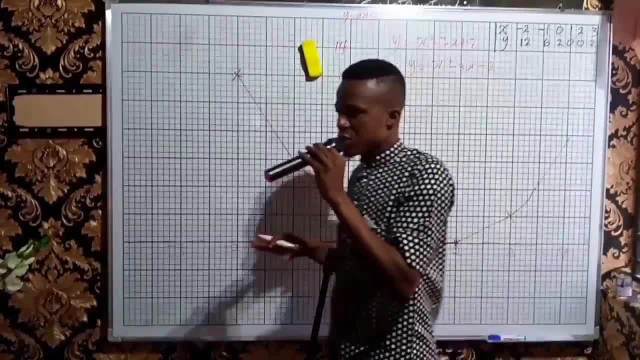 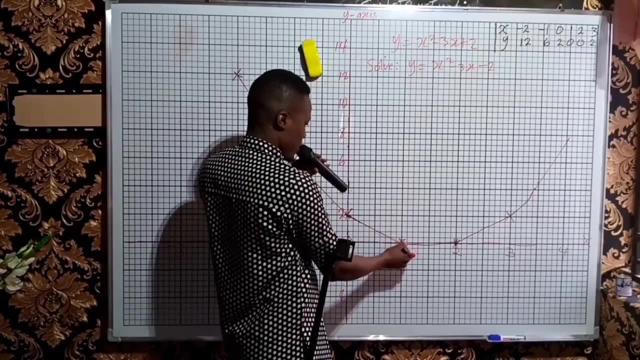 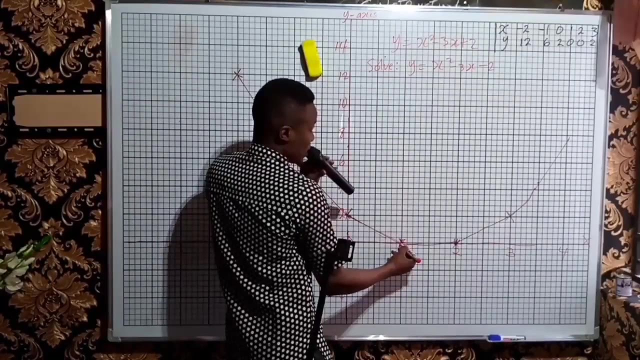 equation. the root of a quadratic equation is obtained from the graph at the point where the curve is uh touching the points where the curve is touching the x-axis. as you can see clearly here, the curve is touching the x-axis as two different points, so the roots of the equation. 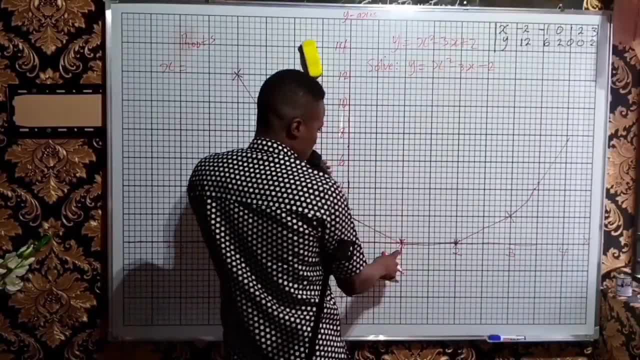 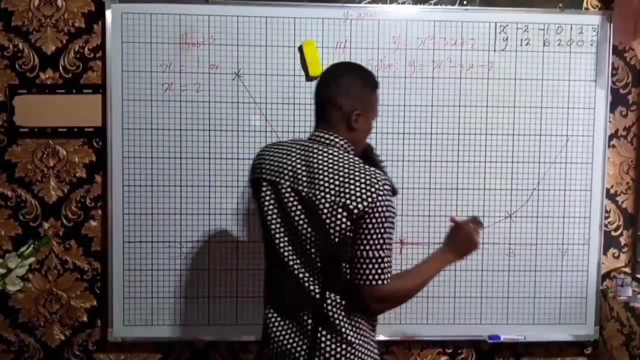 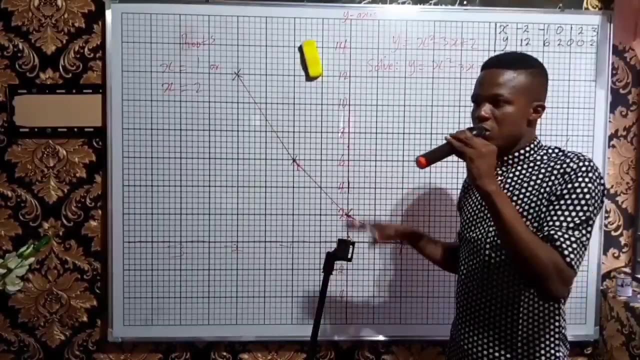 our roots will now be x equal to. is touching it at point one or at point two? so x is equal to two or one. these are the roots of the quadratic equation. so to get the roots of a quadratic equation, only use the two points where the curve is touching the 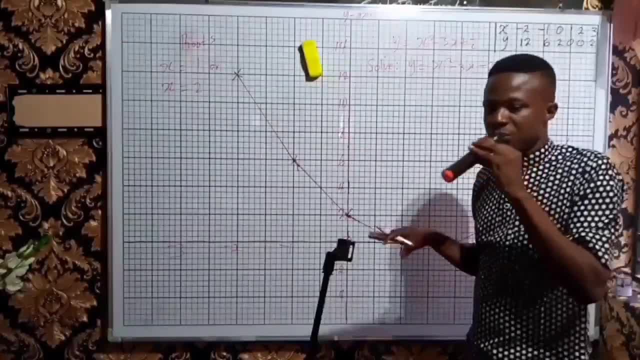 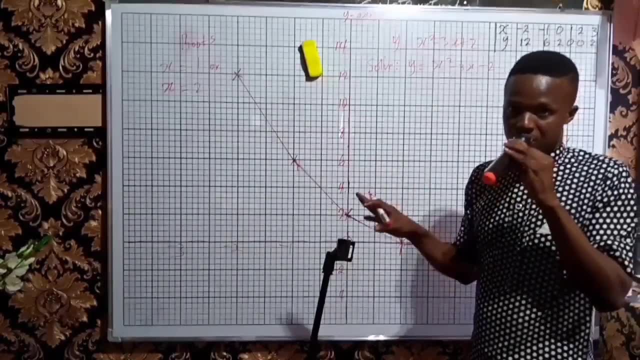 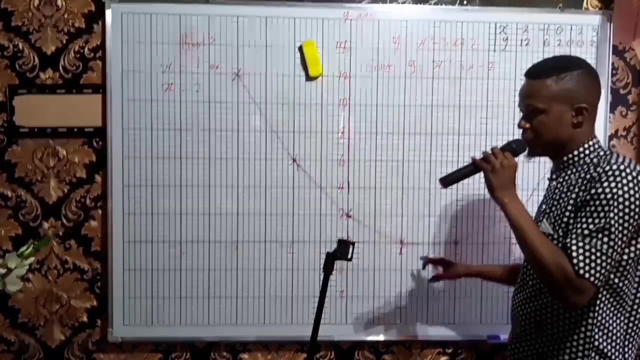 x-axis. sometimes, like i said in the beginning of this video, that the curve can touch the x-axis at point one. okay, that in that case it means that the roots are real but equal. well, this time around we'll find out that the roots are real but distinct. two different values in quadratic equations: curve: 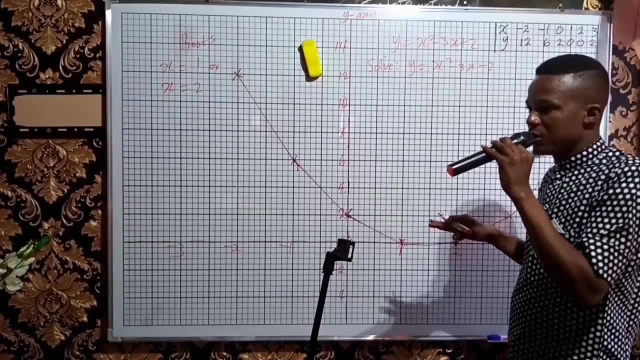 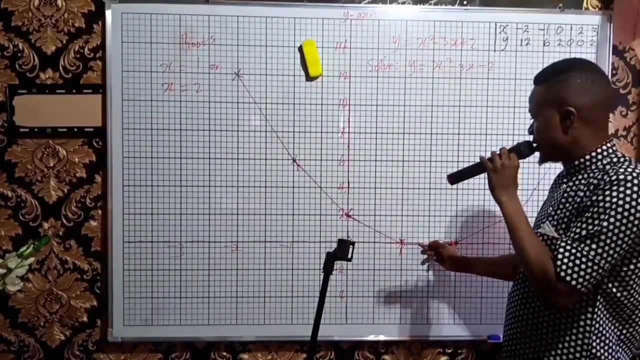 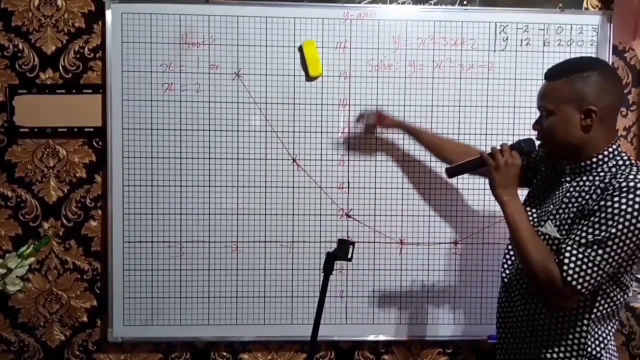 or graph. you can also be asked to get either the minimum or maximum values of x and the values of y. here this is lying at the origin. so the minimum value of x- here this is the minimum- is lying at 0. okay, but if the curve is upside down, it's going to have a maximum value this time around, since 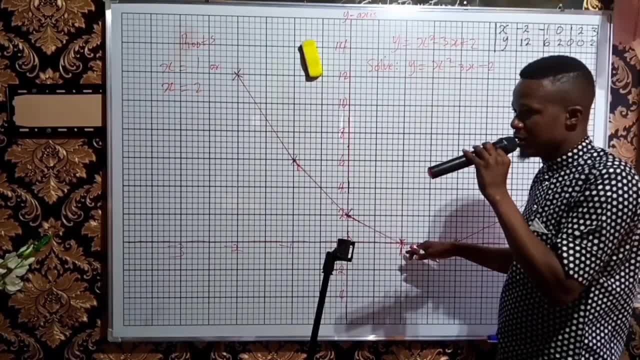 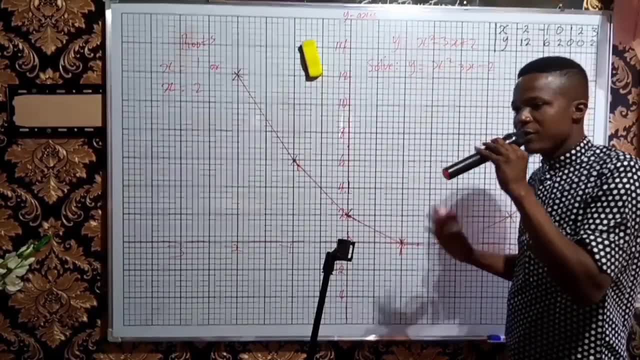 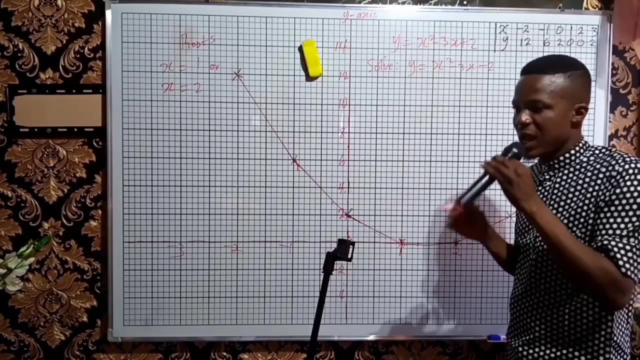 it is like a curve shape, the car will have a minimum value. okay, so there are two cases: it can have a minimum value or a maximum value, but the question we have today does not require us to get a minimum or maximum value, because it was not part of the questions that is asked. 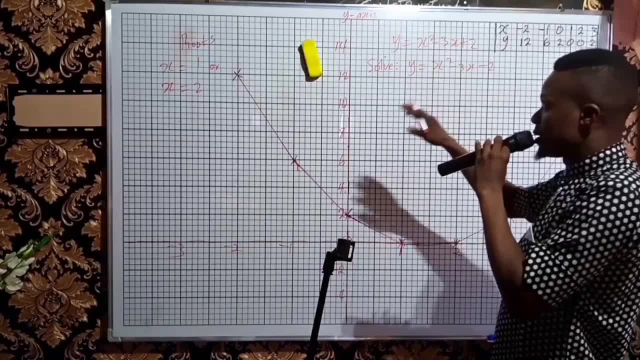 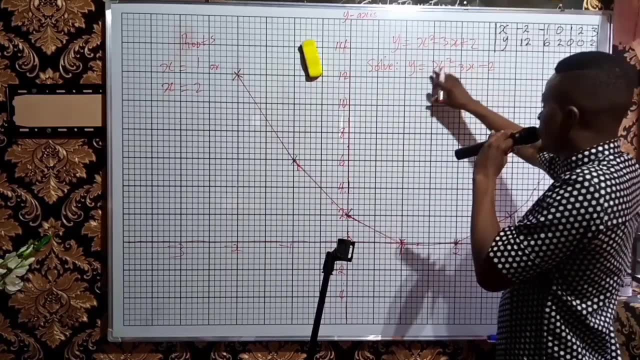 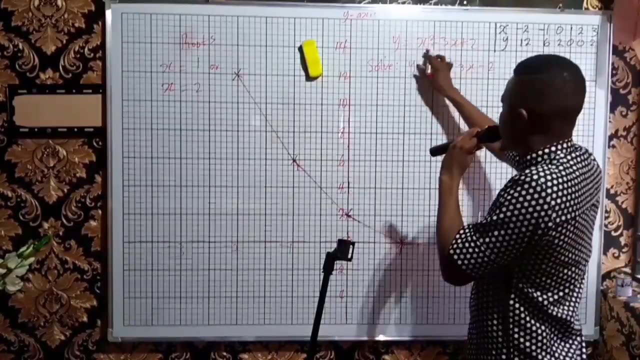 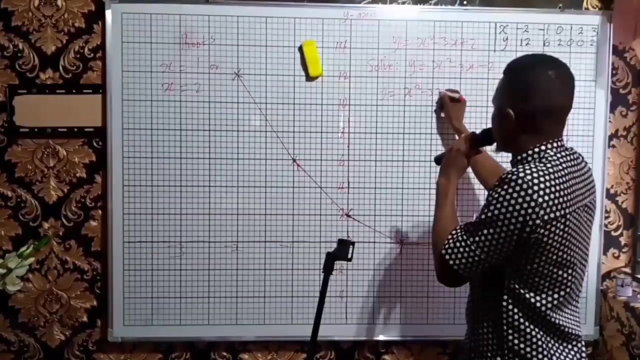 okay, um, at this point we've successfully got the roots of the quadratic equation. let us not answer this question, because we are asked to solve this given quadratic equation from the graph. okay, now to solve this. from the graph, you see that y is x squared minus 3x plus 2. you can see say that y equals x squared minus 3x plus 2. 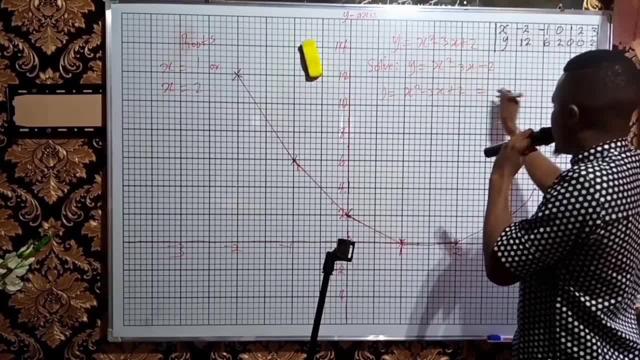 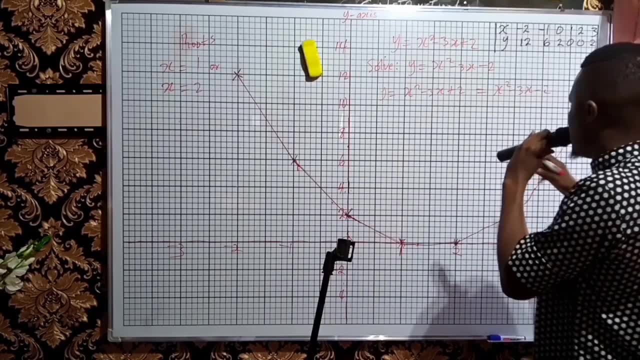 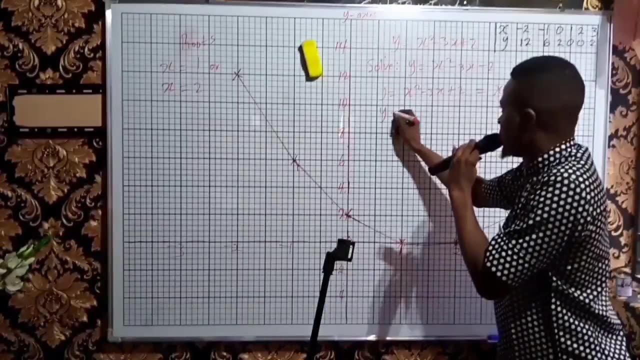 equal to this same value, because this value is, uh, x squared minus 3x. okay, then, having done that, the next thing you do is to collect light terms or to bring this value into the right hand side, so you have that y is x squared, this one coming in, or to be faster. 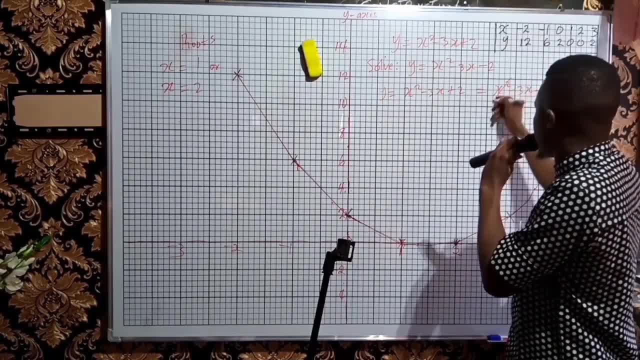 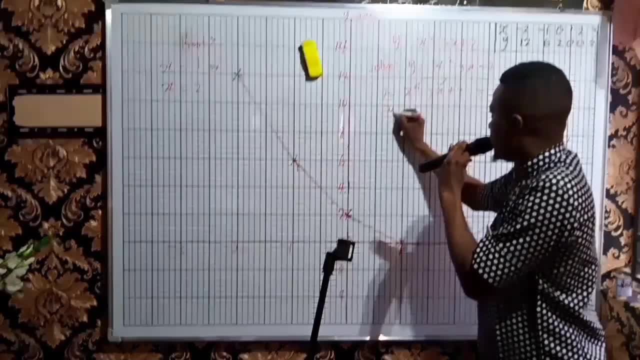 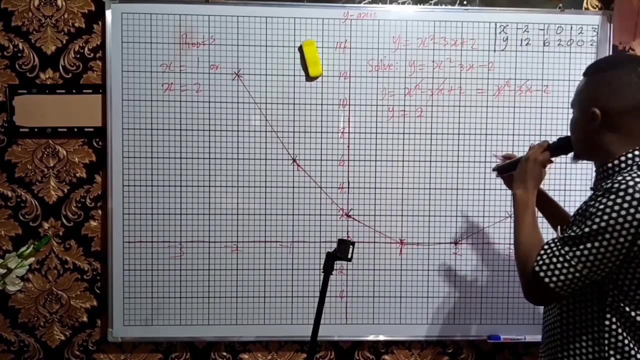 what you just need to do here is to say: um x squared, you cancel x squared minus 3 coming here is plus it cancels out. we only have um y equals 2. 1 minus 2. that is here is crossing over. the minus 2 must change into plus 2.. okay, so you have y equals 2 plus 2. 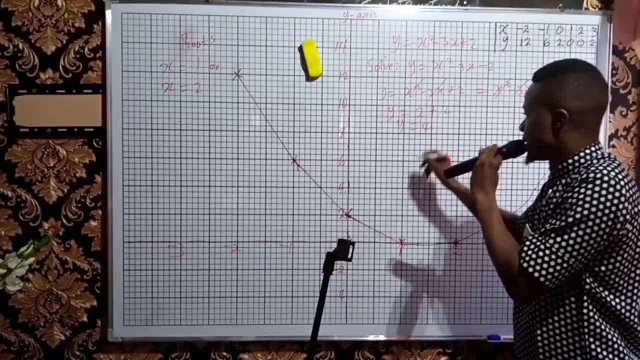 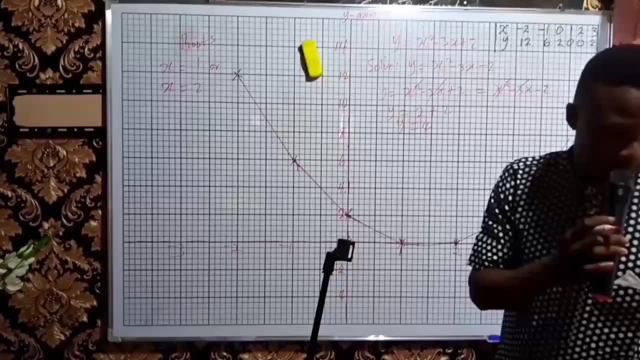 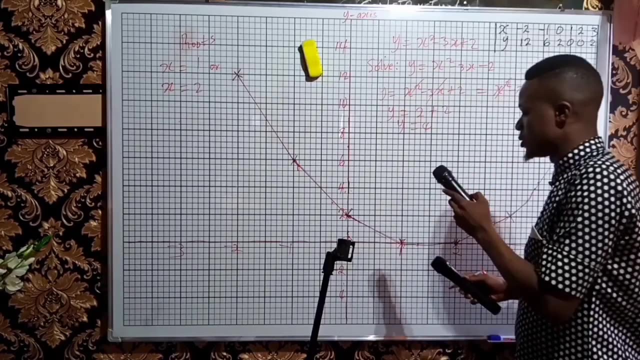 and 2 plus 2 will give us uh 4. that is the value of y. then, having got 4 as the value of y, you need to plot in 4 for the value of y. so draw a line: y equal to 4. that is what you are required to do here. 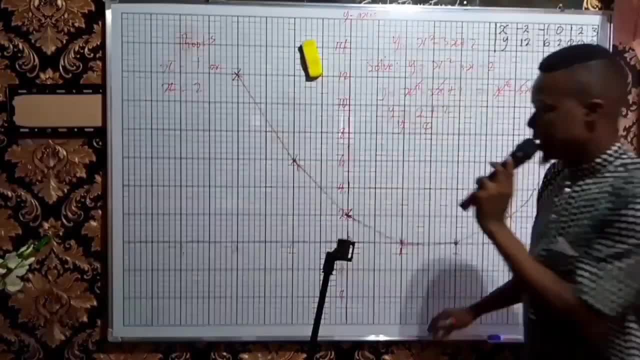 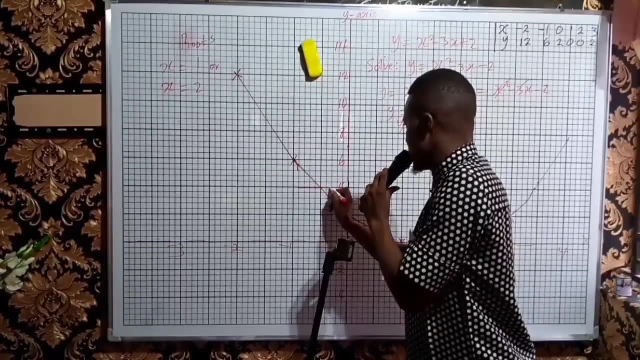 you must draw a line of y equal to 4.. and how do you do that? this is where y is four, so use your ruler. i may not use ruler here, but when you're doing it in exam, usually to draw a straight line at that point where your y. 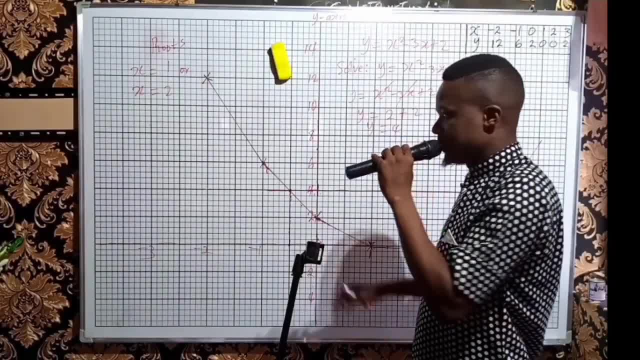 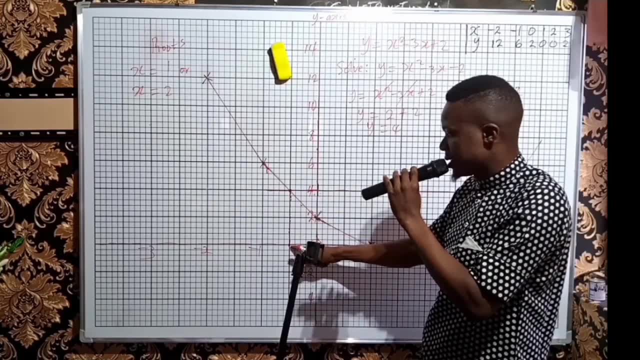 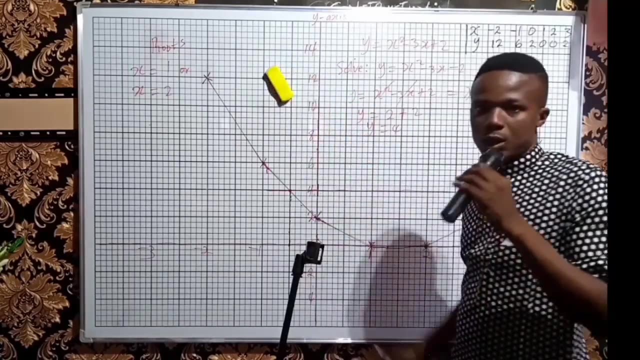 is equal to four. okay, at this point, after you must have drawn the straight line and trace down here, the point where this line is touching the x axis will be part of the solution. okay, i haven't drawn the straight lines and traced down the point. we are these line you've 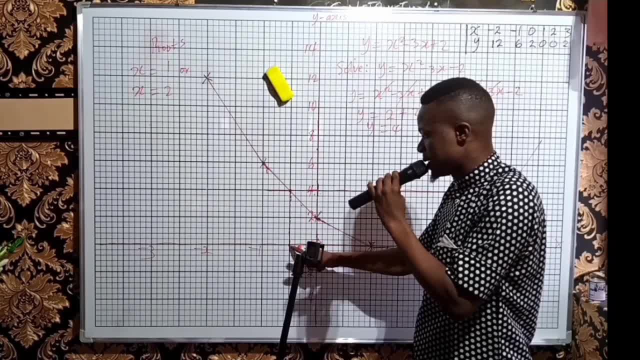 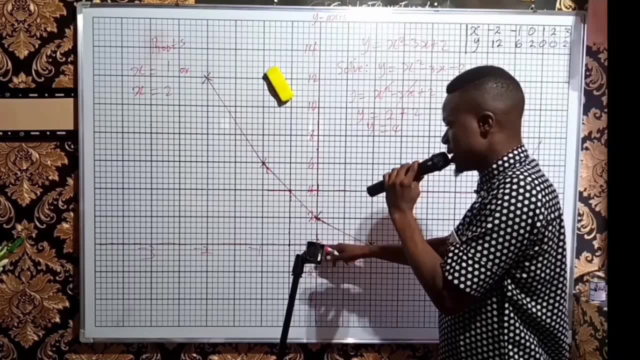 drawn down here is touching the x-axis will be part of the solutions to this given quadratic equation. you can see that the first point here is 0, 0.1, 0.2, 0.30, 0.4, 0.5, so um part of the values of 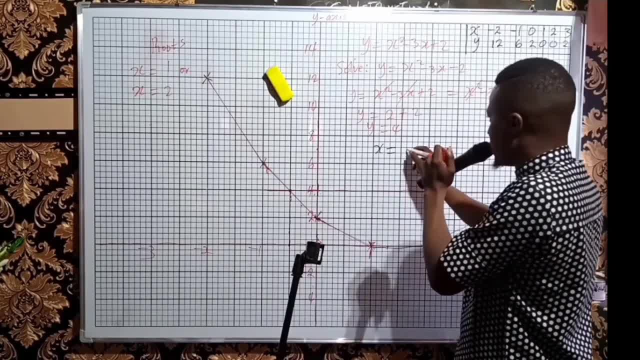 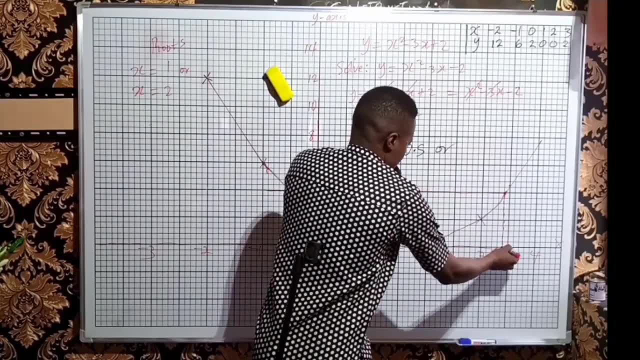 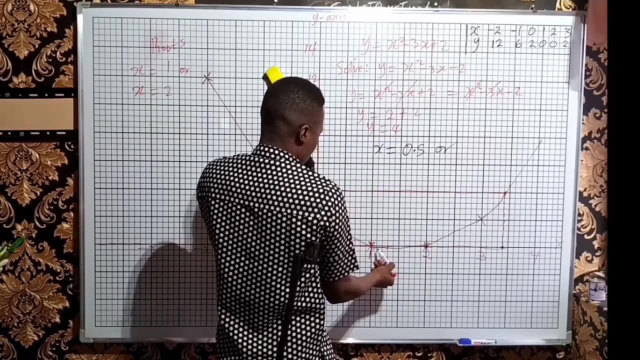 x to the solution of this quadratic equation is 0.5. that means we have a solution that is. Or look at another point where it's fortunate At this point here. here it's 3, each small box is 0.1, since you are counting in 1 and there are 10 openings. 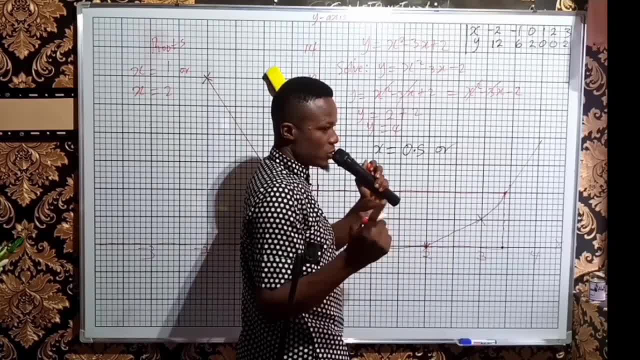 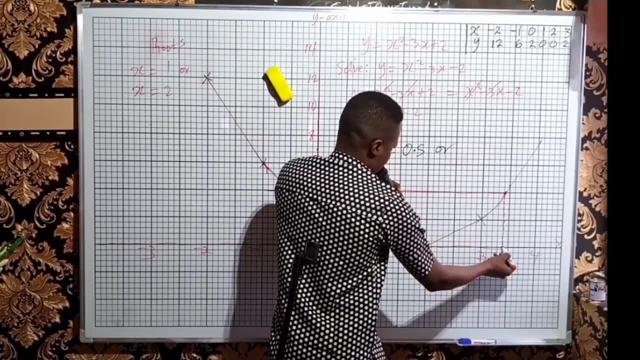 10 divided 1 divided by 10 will give us 0.1. So every small box is 0.1.. So if here it's 3, we have 3.1, 3.2, 3.3 and 3.4.. 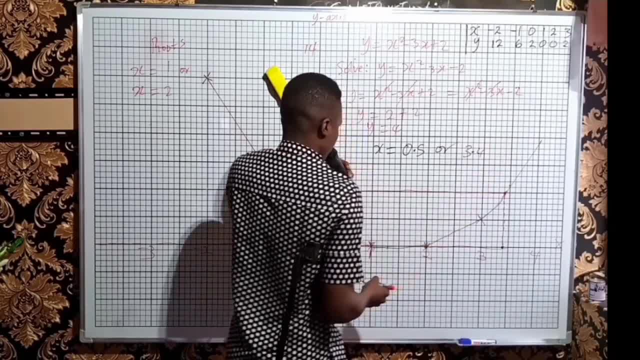 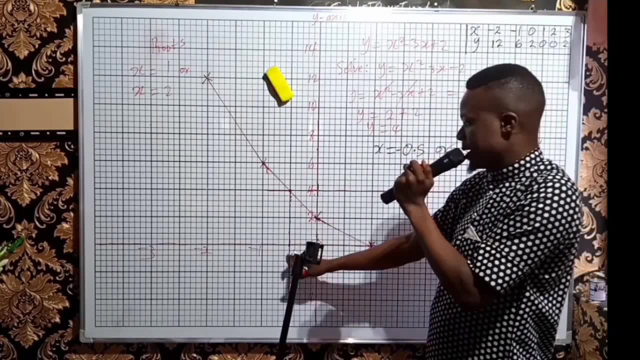 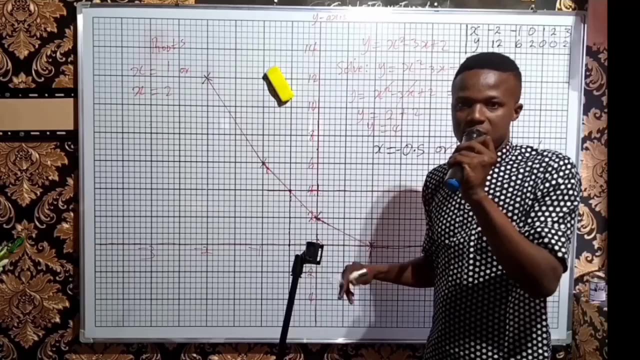 So you see that the values of x can be 0.5, minus 0.5, because that is the negative side. We have minus 0.5, here it's negative, while here it's positive. Minus 0.5 or 3.4 is not the roots of the quadratic equation they want us to solve from the graph. 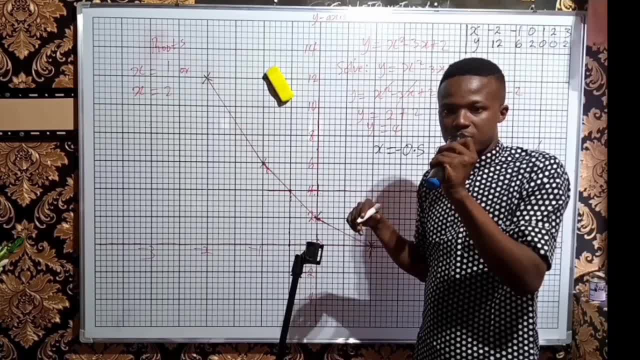 Okay, thank you so much for your audience. Kindly hit the red button to subscribe to my channel if you enjoyed what you've watched. Thank you.